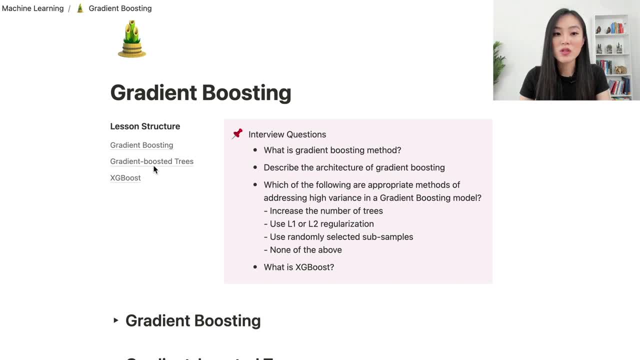 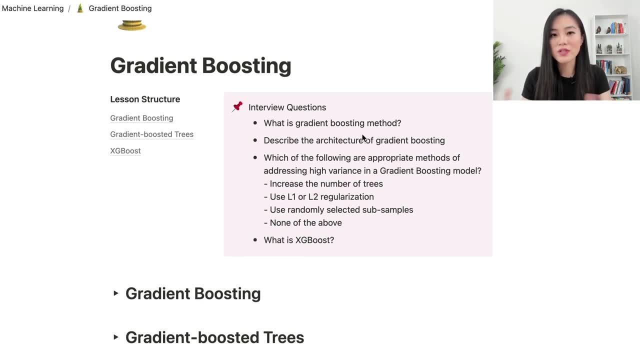 and then we'll look at what is gradient boosting, what are gradient boosted trees and finally we'll talk about actually boost. Okay, let's start with looking at some interview questions to give you a sense of what are the questions you might get in interviews. 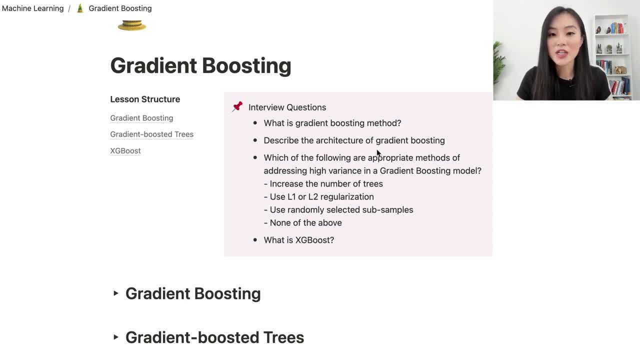 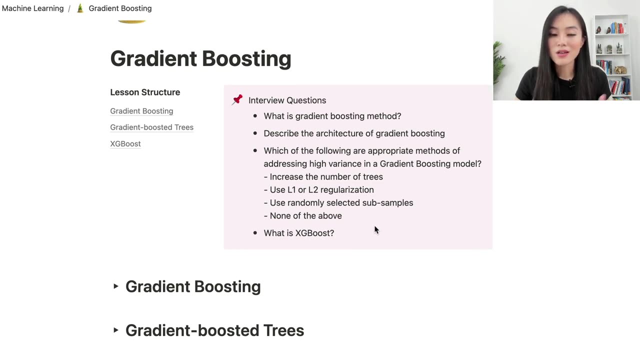 What is gradient boosting methods? Describe the architecture of gradient boosting. Which of the following are appropriate methods of addressing high variance in a gradient boosting model? Increase the number of trees. use L1 or L2 regularization. use randomly selected subsamples. none of the above. What is actually boost? 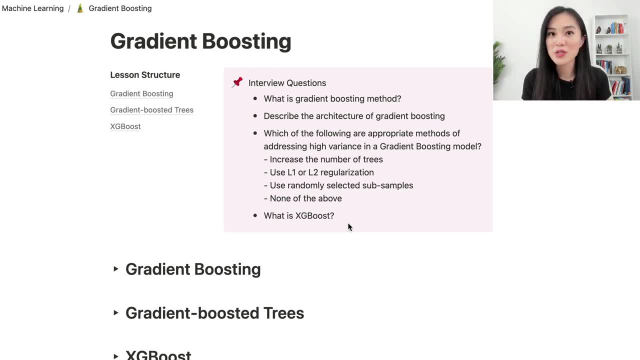 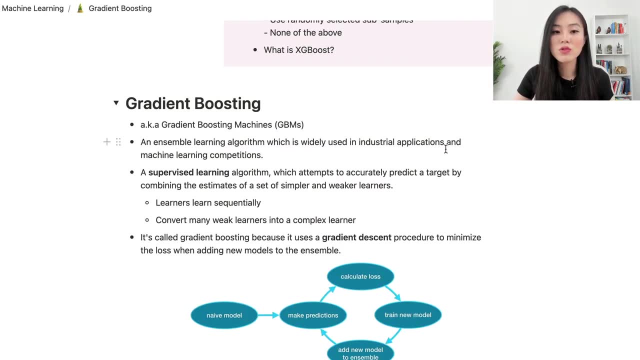 After watching this video, you should be able to answer all these interview questions. Alright, let's dive in. Okay, let's start with learning about gradient boosting. Gradient boosting is also known as gradient boosting machines or GBMs. It's an ensemble. 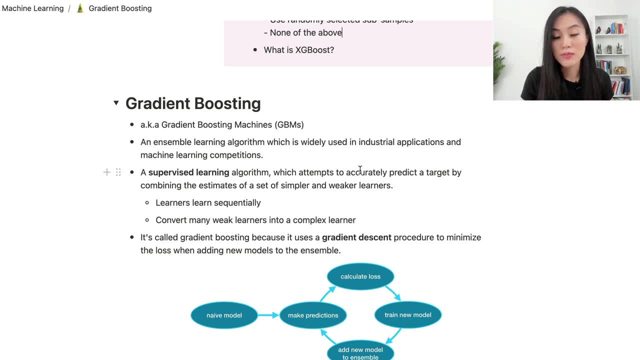 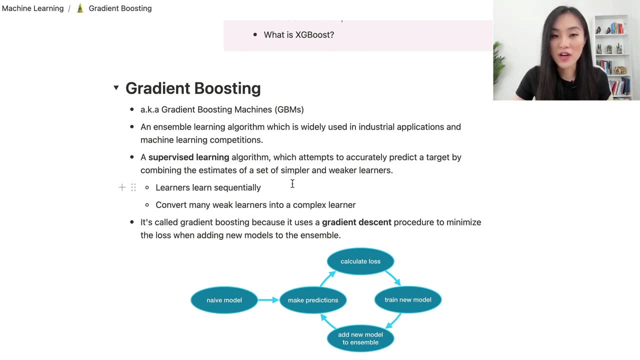 learning algorithm which is widely used in industrial applications and machine learning competitions. as I mentioned earlier, It's also a supervised learning algorithm which attempts to accurately predict a target by combining the estimates of a set of simpler and weaker learners. These weaker learners learn sequentially and the algorithm 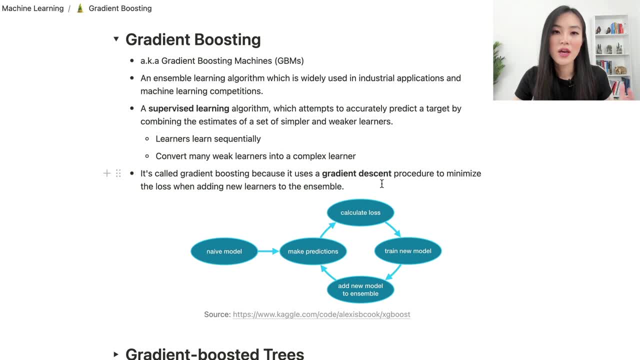 converts many weaker learners into a complex learner. It's called gradient boosting because it uses a gradient descent procedure to minimize the loss when adding new learners to the ensemble. Here's a diagram showing how it works. We start with a naive model or a simple model. 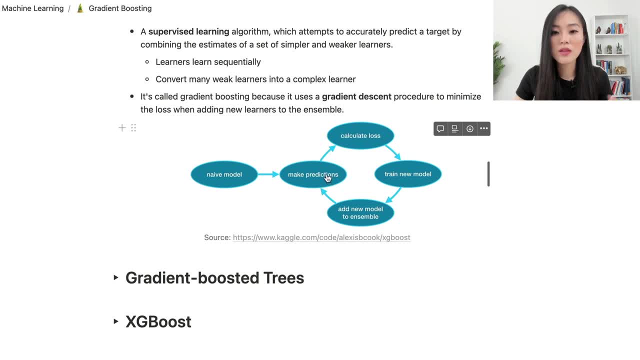 Then we use this naive model to make predictions. Once we get the predictions, we can calculate the loss based on the loss function, And then we train a new model based on the loss we calculated from the previous prediction, And then we add this new model to. 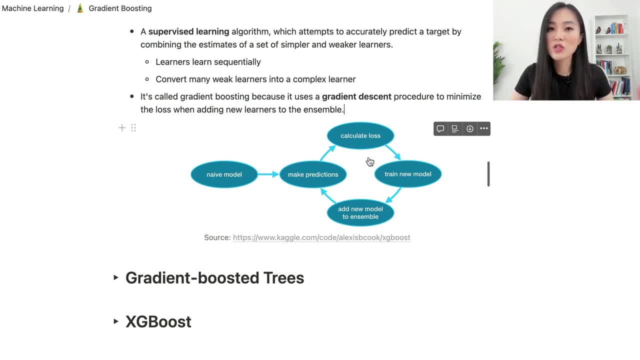 the ensemble, we make predictions again. So you can see that it's an iterative or sequential process and we keep adding new models to the ensemble and the predictions will be improved. Okay, now we have a basic idea of how gradient boosting works. Let's look at gradient boosted. 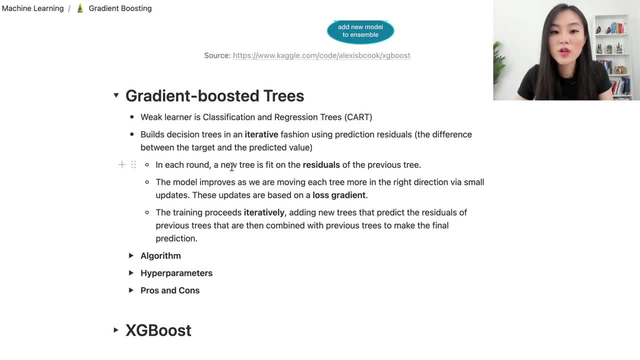 trees. Gradient boosted trees is a gradient boosting algorithm. when the weak learner is classification and regression trees, or CART. It views decision trees in an iterative fashion using prediction residuals, which is the difference between the target and the predicted value. In each iteration, a new tree is fit on the residuals of the previous tree. 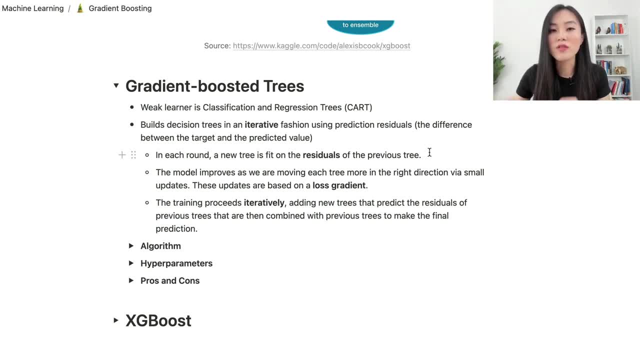 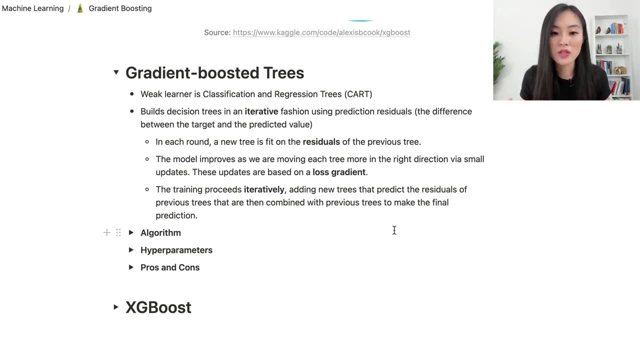 Then the model improves as we are moving each tree more in the right direction via small updates. These updates are based on a loss gradient, The training process, iteratively adding new trees that predict the residuals of previous trees that are then combined with previous trees to make the final prediction. Now let's look at the algorithm in detail. Sometimes you might get 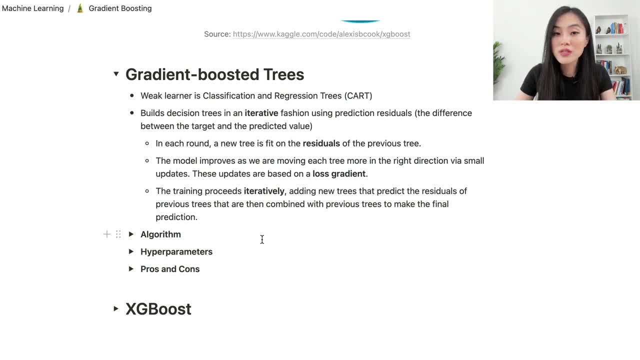 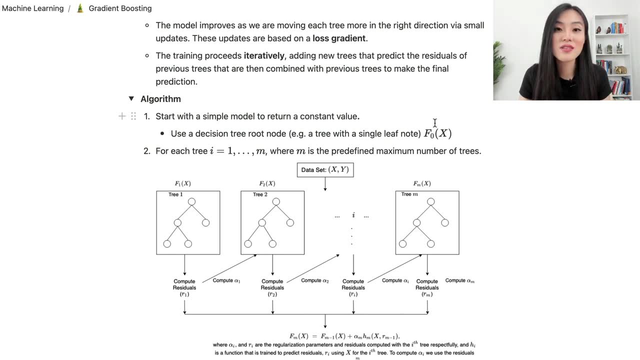 interview questions about the architecture of gradient boosted trees. so it's helpful for you to know how the algorithm works step by step. So we start with a simple model to return a constant value. We start using a decision tree root node, a tree with a single leaf node. 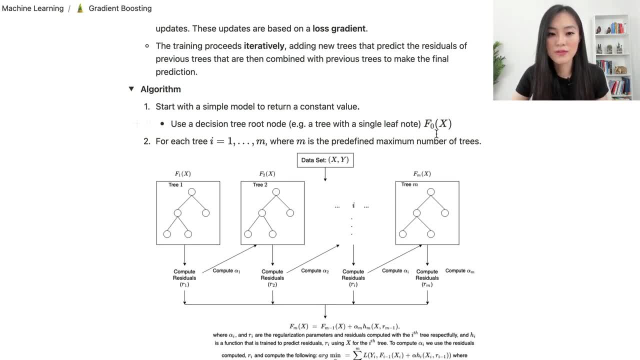 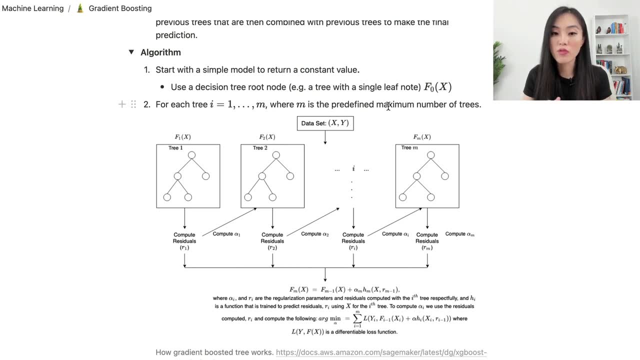 as the first model, Let's call it F0x. For each tree i from 1 to m, where m is a predefined maximum number of trees or maximum number of iterations, there are a few things we need to do. We first compute the residual Ri of that tree and then we calculate the learning rate, alpha, Based on the. 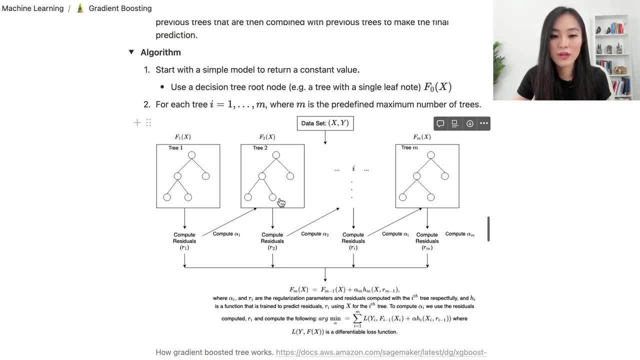 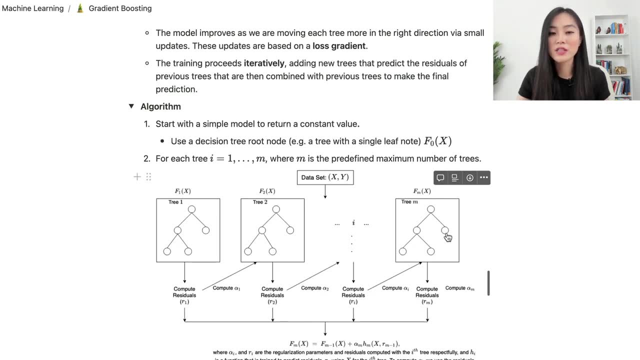 residuals and alpha. then we build a new tree, Then we add this new tree to the ensemble and then we continue the next iteration to build new trees and finally we combine the predictions of all trees to output the final prediction. That's a general idea of how it works. Now let's 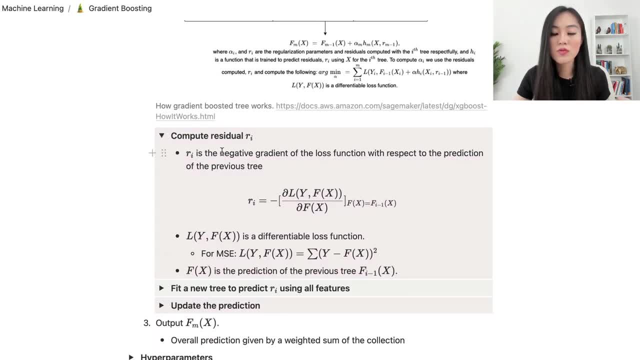 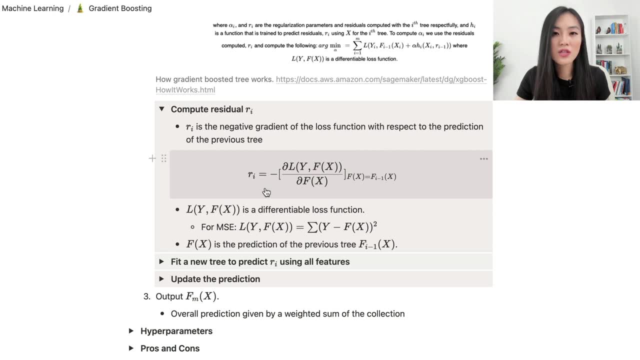 look at each step in detail. We first compute the residual. Ri Ri is a negative gradient of the loss with respect to the prediction of the previous tree. Here's the equation of Ri Ri is a negative value of the partial derivative of the loss function. Ly with respect to Fx, which is the 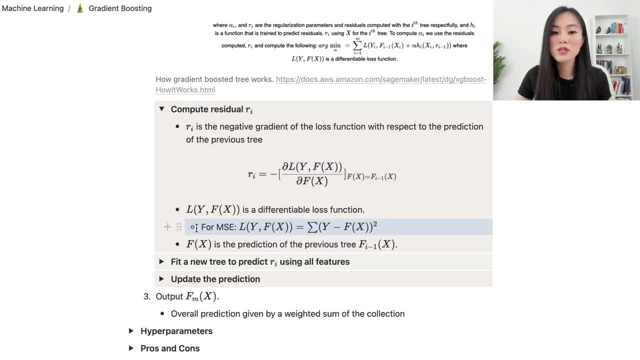 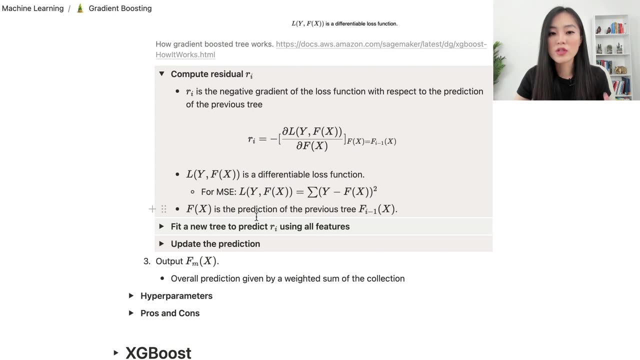 prediction of the previous tree. For example, if we are using mean squared error for the loss function, then our loss function, Ly, is the sum of squares of the difference between y and Fx. y is the actual label and Fx is the predicted value. Once we have the residual, 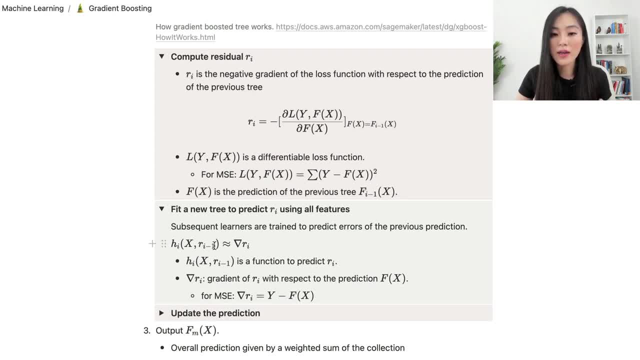 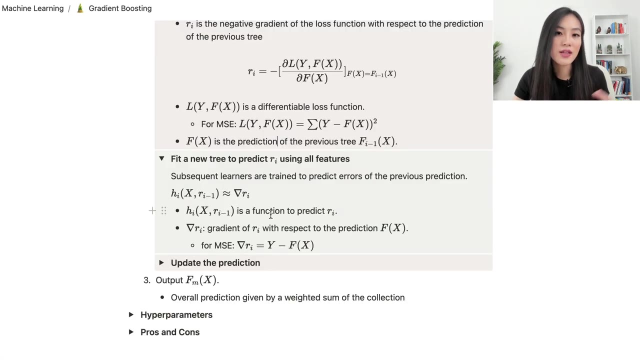 Ri, then we fit a new tree to predict Ri using all the features available to us. The idea is that subsequent learners are trained to predict errors of the previous prediction. So our model will be improved because we keep correcting our previous mistakes And let's say, hi is a function. 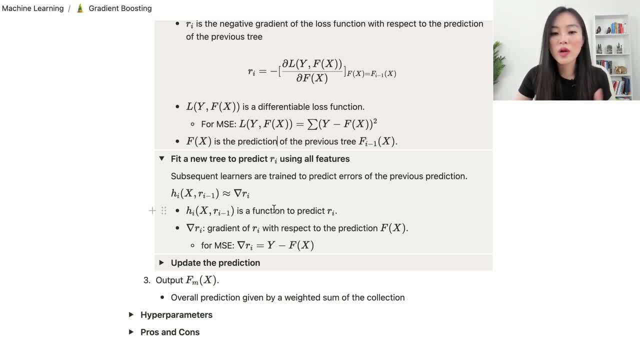 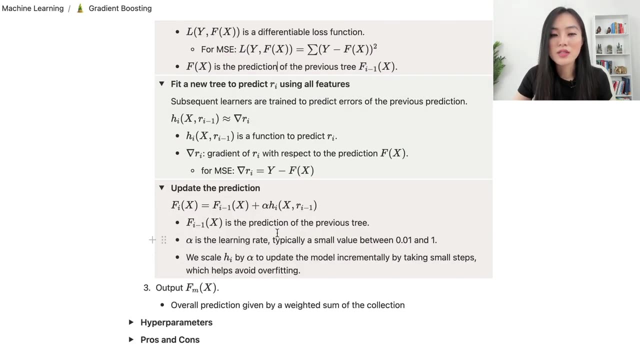 to predict Ri. So this function is similar to the gradient of Ri. with respect to the prediction Fx, If we have the error loss, then the gradient of Ri is precisely the residual the difference between y and Fx. The next step is simply to update the prediction. Our new prediction in iteration i: 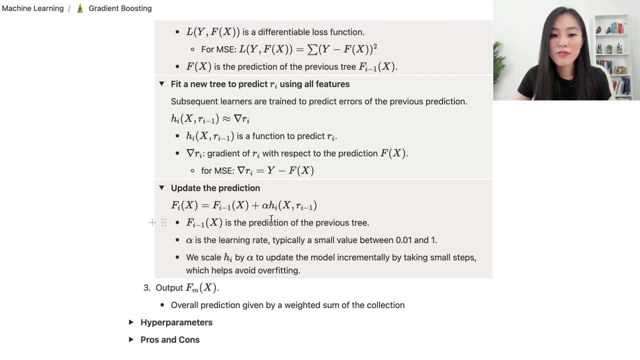 will be the prediction of the previous tree plus alpha multiplied by hi. Alpha is the learning rate, typically a small value between 0.01 and 1.. And here we scale hi by alpha to update the model incrementally by taking small steps, which helps avoid the error loss. So if we have the error loss, 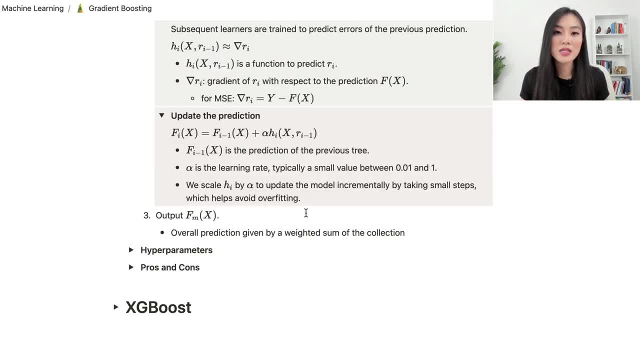 then the gradient of Ri is precisely the residual, the difference between y and Fx, And here we scale hi by alpha to update the model incrementally by taking small steps, which helps avoid overfitting. Finally, once we reach the maximum number of trees or the number of iterations, 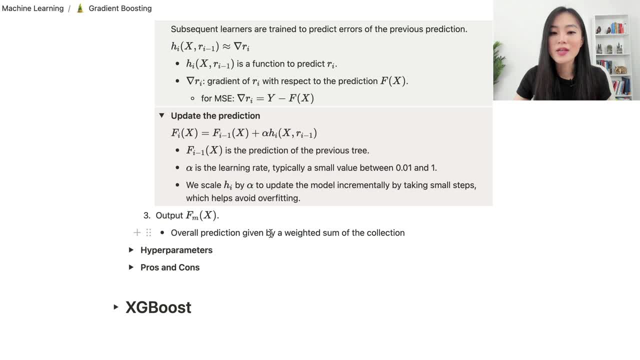 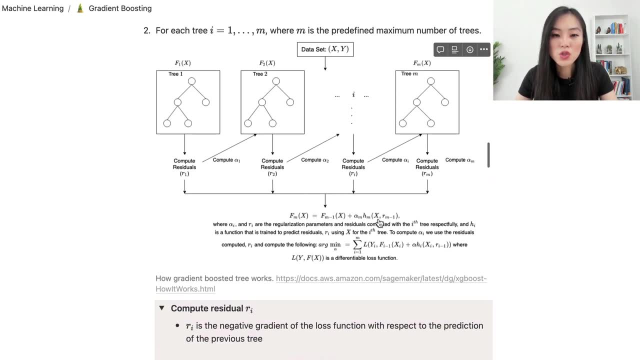 then we output Fmx. the overall prediction is given by a weighted sum of the collection. So these are the three steps of the algorithm. If you got an interview question about the architecture of gradient boosting or gradient boosted trees, then you should be able to draw. 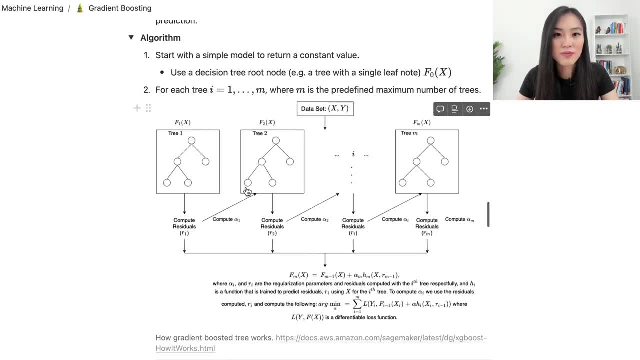 this diagram and explain what happens in each iteration. Okay, now let's move forward to the high-properimeters of gradient boosted trees. Now let's move forward to the high-properimeters of gradient boosted trees. Now let's move forward to the high-properimeters of gradient boosted trees. 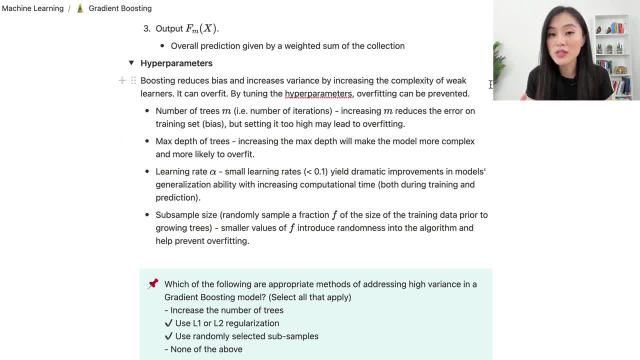 Boosting reduces bias and increases variance. by increasing the complexity of weak learners It can overfit And by tuning the high-properimeters overfitting can be prevented. Here are the high-properimeters we can tune. The first one is number of trees: M. 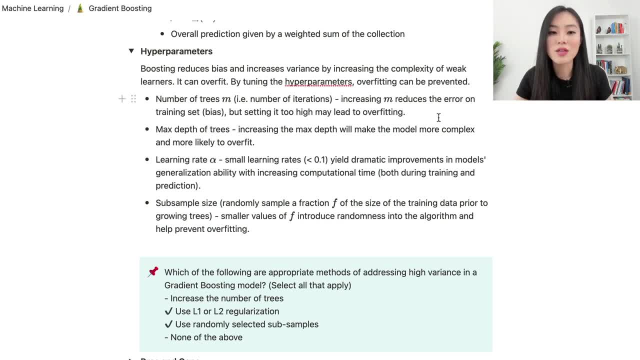 or the number of iterations. Increasing M reduces the error on the training set, so it will reduce the bias. But setting too high may lead to overfitting. Maximum depth of trees is another high-properimeter we can tune. Increasing the maximum depth will 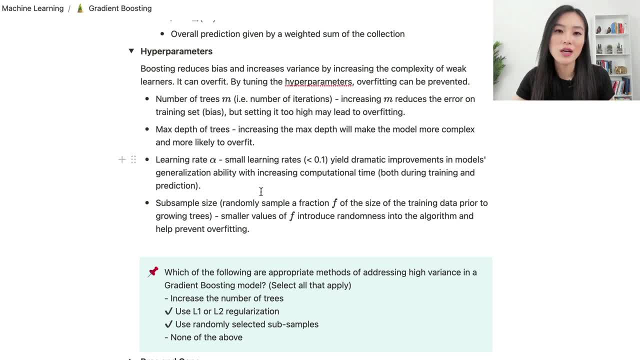 make the model more complicated and more likely to overfit. Another high-properimeter we can tune is the learning rate alpha. Small learning rate- when alpha is less than 0.1, yield a dramatic improvement in the model's generalization ability. But small learning rate means increasing. 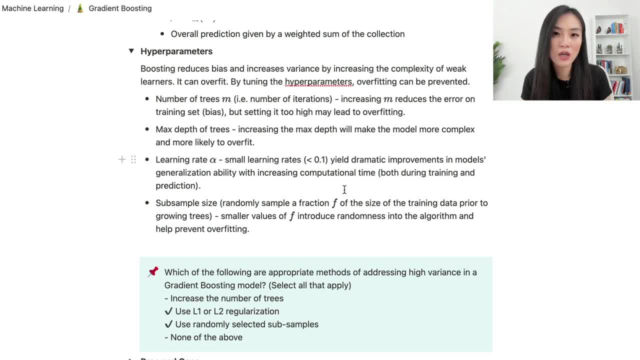 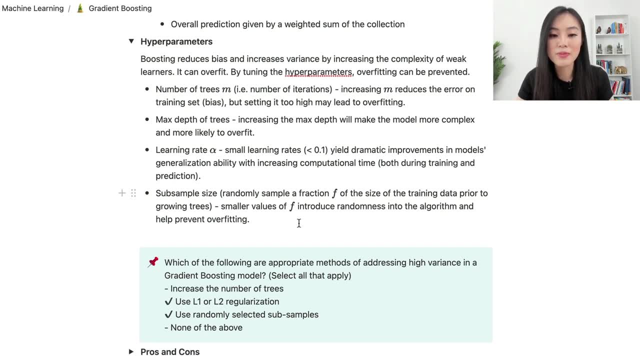 commutational time, both during training and prediction. So there's a trade-off we need to make when you find the optimal learning rate for our dataset. Another high-properimeter is the sub-sample size. We randomly sample a fraction of our data set. We randomly sample a fraction of 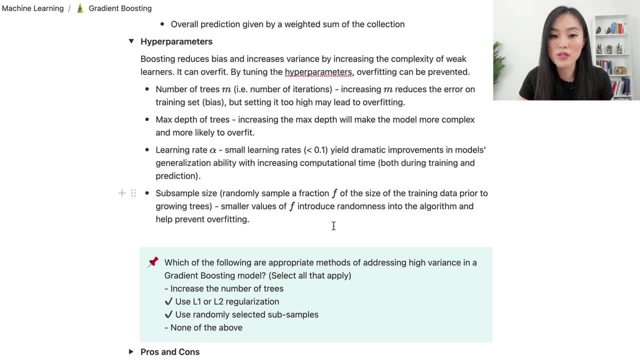 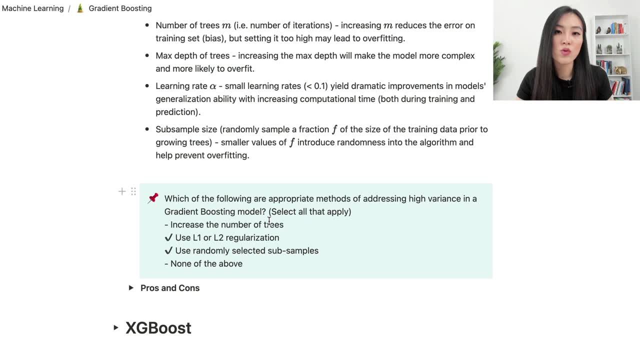 the size of the training data prior to growing trees. Smaller values of f introduce randomness into the algorithm and help prevent overfitting. Now let's look at one of the interview questions we mentioned at the beginning of this video. Which of the following are appropriate methods? 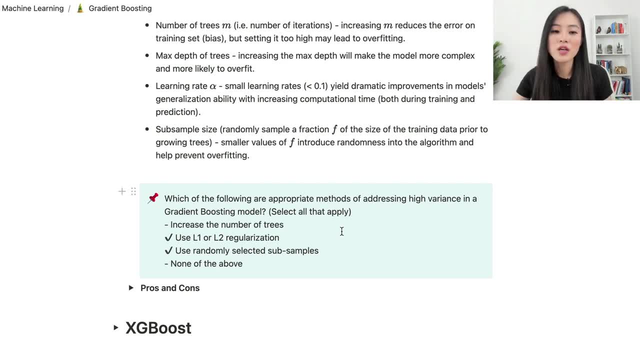 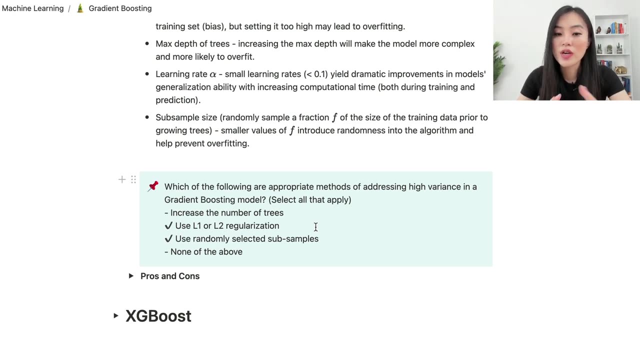 of addressing high variance in a gradient boosting model. The first one is increase the number of trees. Increasing the number of trees will not help prevent overfitting. In fact, it will lead to too high variance. The second choice is to use L1 or L2 regularization. This will help prevent 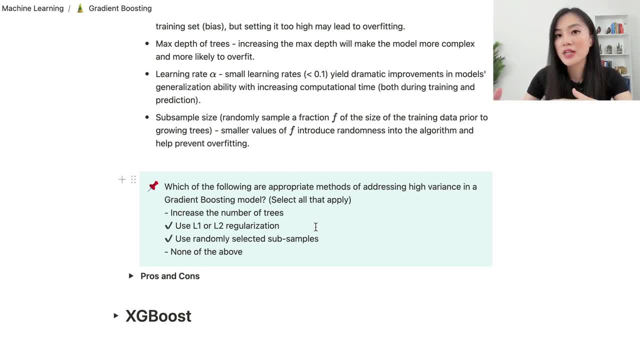 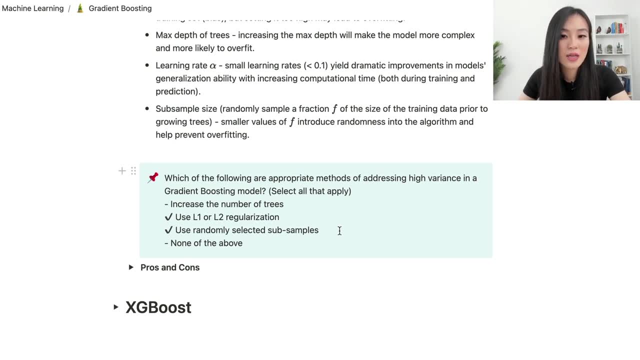 overfitting, because adding regularization term is basically adding a penalized term to the loss function. The next choice is to use randomly selected sub-samples, As I mentioned earlier, when we select a sub-sample from the training data, we introduce randomness to the algorithm. 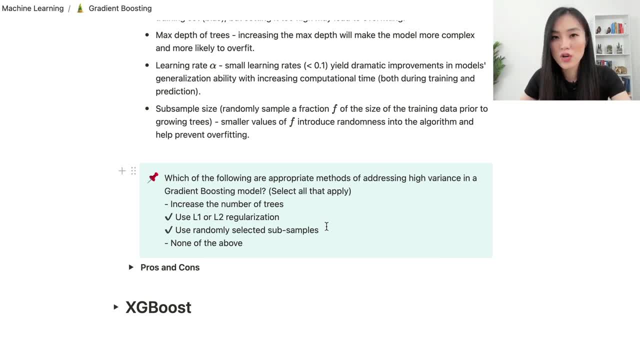 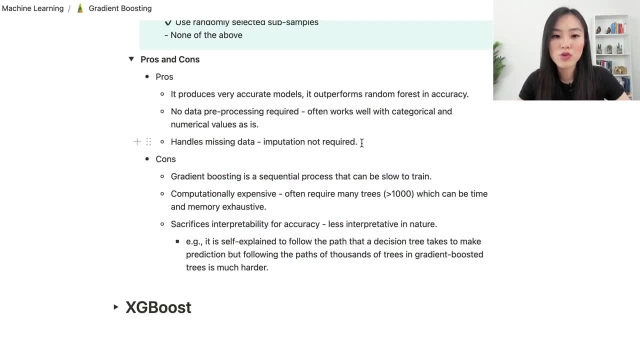 and that will help prevent overfitting. So the second choice and the third choice will be the right answer to this question. Now let's summarize the process Cons of gradient boosted trees. Gradient boosted trees have some advantages. It produces very accurate models and often it outperforms random forest in accuracy. There is no data pre-processing. 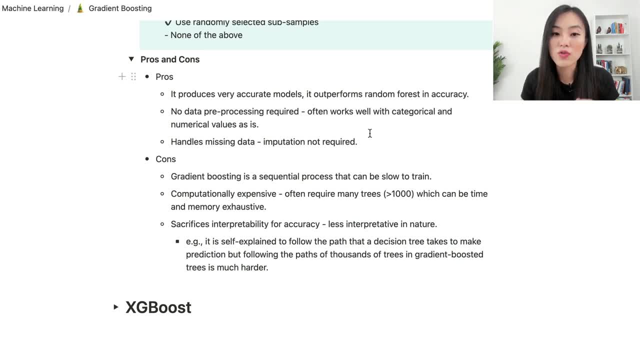 required. It often works well with categorical and numerical values, as is. It can also handle missing data well. Imputation is not needed before we fit the data into the model. There are also some downsides of gradient boosted trees. Gradient boosting is a sequential process that can be. 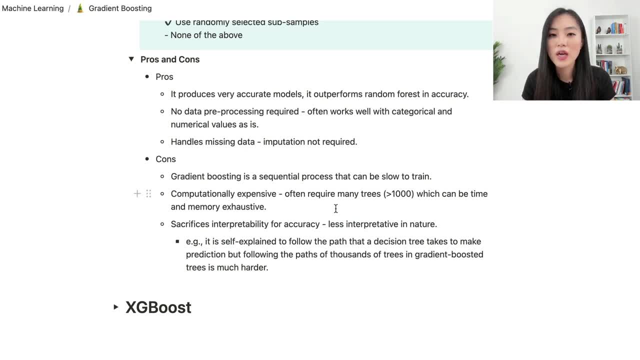 slow to train. It's also computationally expensive. It often requires many trees, over a thousand, which can be time and memory exhaustive. Another downside of gradient boosted trees is that it sacrifices interpretability for accuracy. It's less interpretative in nature, For example. 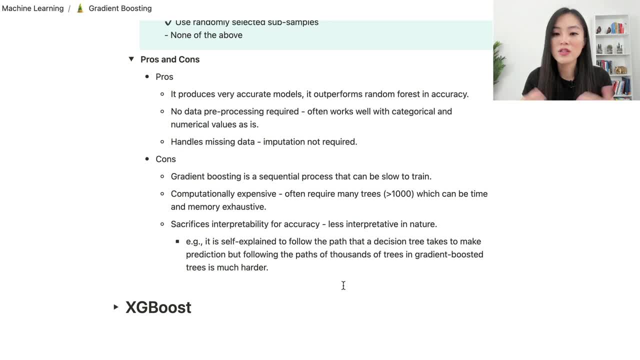 it is self-explanatory to follow the path that the decision tree takes to make prediction, But following the path of thousands of trees in gradient boosted trees is much harder, So in terms of interpretability it's not as good as decision trees. 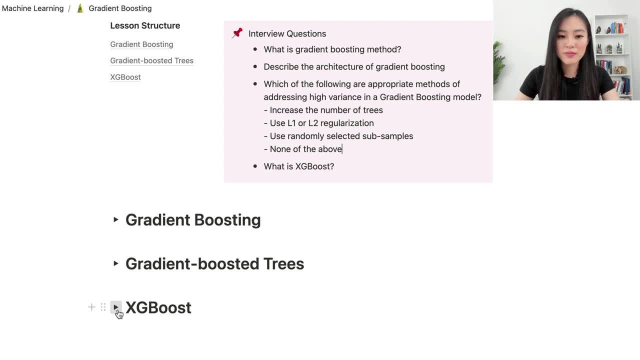 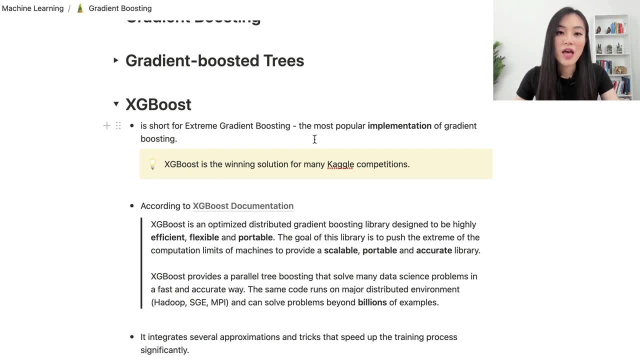 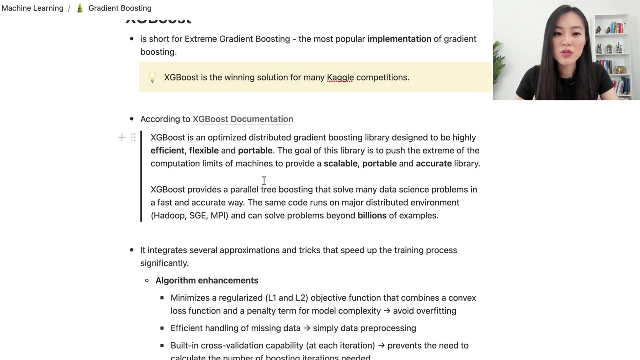 Finally, let's talk about XGBoost. What is XGBoost? XGBoost is short for extreme gradient boosting. It's the most popular implementation of gradient boosting. XGBoost is also the winning solution for many Keiko competitions. According to its documentation, XGBoost is an optimized